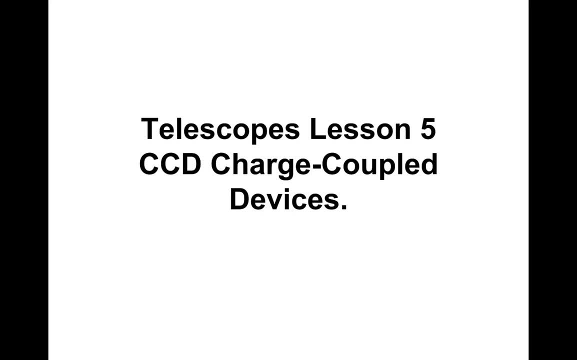 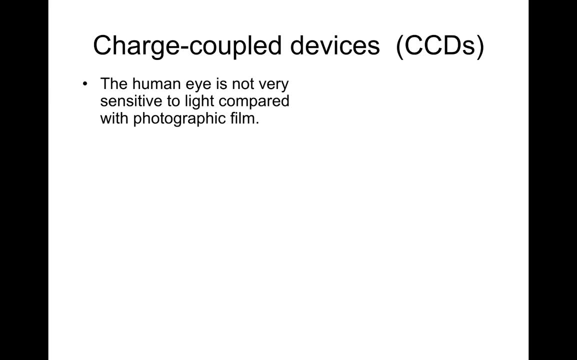 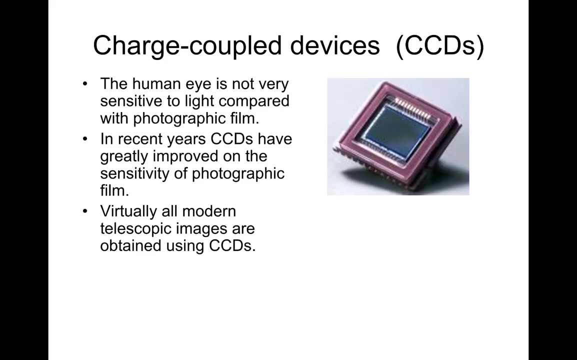 Hello, this is Astrophysics Telescopes, Lesson 5, and this is CCD, or Charged Coupled Devices. So the human eye is not very sensitive to light compared with photographic film, and in recent years CCDs have greatly improved on the sensitivity of photographic film and virtually all modern telescopic images are obtained using CCDs. 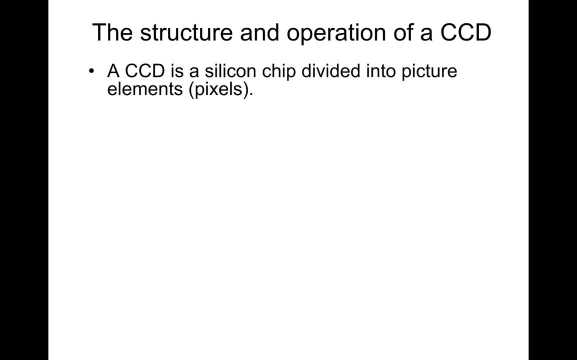 So let's look at the structure and operation. So it's a silicon chip divided into picture elements or pixels, and incident photons cause electrons to be released and the number of electrons liberated is proportional to the intensity of the light. So intensity is basically the amount. It's nothing to do with the individual energy of the incoming photons. 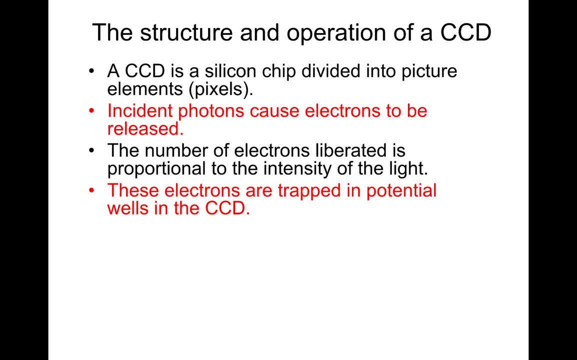 So what happens is these electrons are trapped in potential wells in the CCD And an electron pattern is built up which is identical to the image formed on the CCD, And, when exposure is complete, the charge is processed to give an image. All right, let's move on to quantum efficiency. 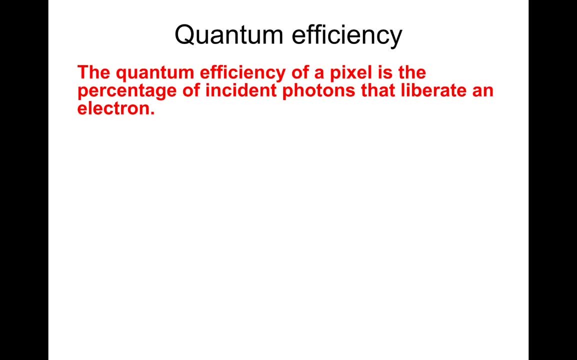 So the quantum efficiency of a pixel is the percentage of incident photons that liberate an electron. So for a CCD this is usually at least 70% and can be up to as high as 90% with certain light wavelengths. When we compare that to photographic film, photographic film is typically 4%. 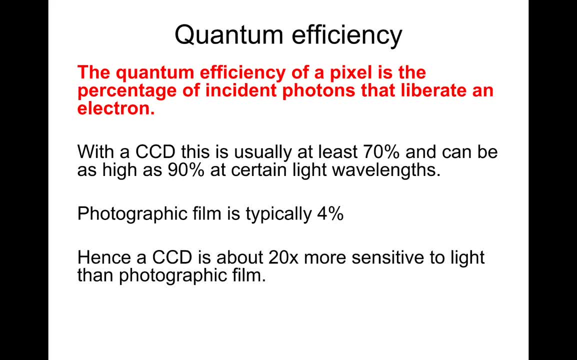 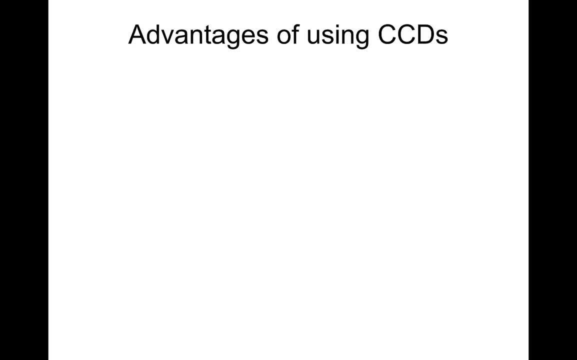 So a CCD is about 20 times more sensitive to light than a photographic film. All right, so some advantages of using CCDs. So they have a much higher quantum efficiency than photographic film. They're therefore far more sensitive to light. 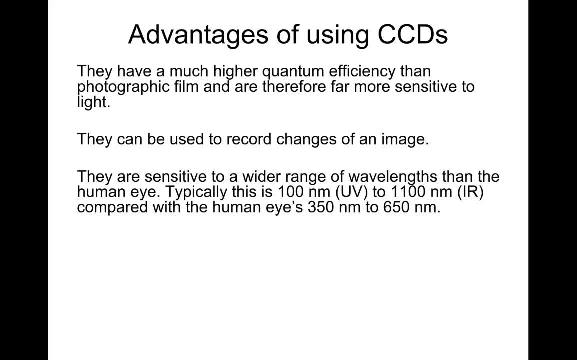 They can be used to record changes of an image. They are sensitive to a wider range of wavelengths than the human eye, Typically between 100 nanometers to 1100 nanometers. so all the way from UV to infrared Human eye is around 350 to 650 nanometers, which is the range of the visible light spectrum. 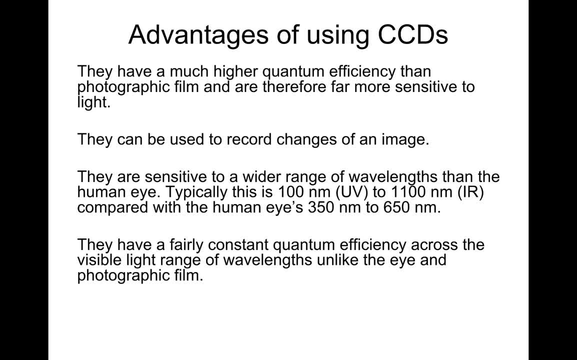 And they have a fairly constant quantum efficiency across the visible light range of wavelengths, Unlike the eye and photographic film. So what I'm going to do now is give you a six mark exam question about CCDs. There's a bit more information in the mark scheme that we've not quite covered, but obviously we're going to go through it anyway, so it doesn't really matter.